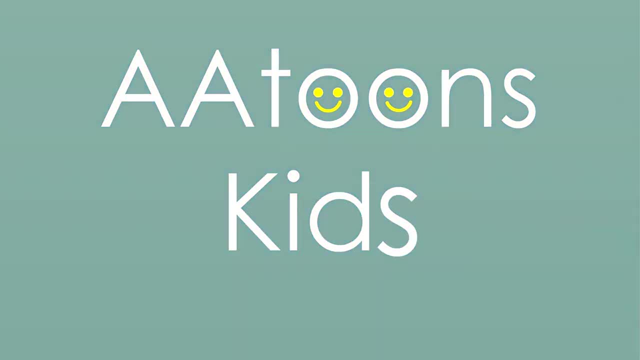 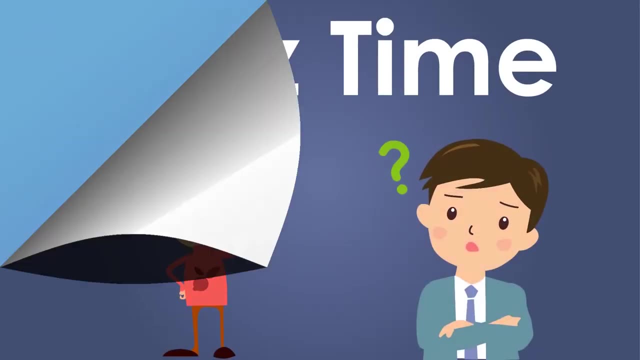 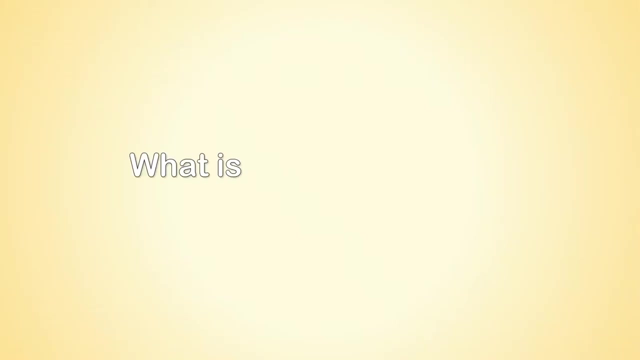 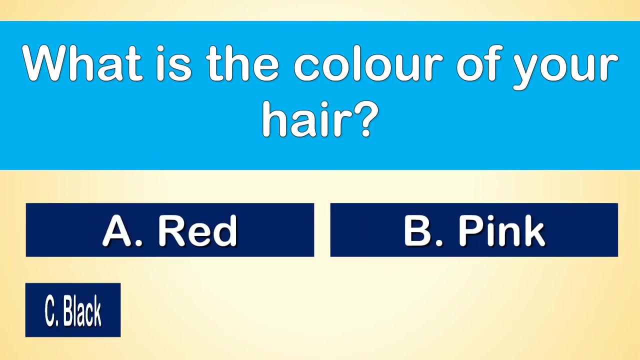 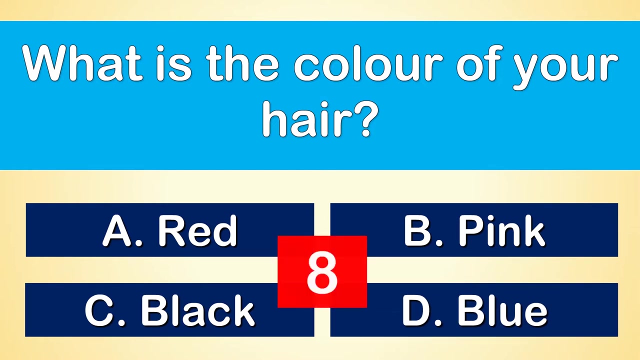 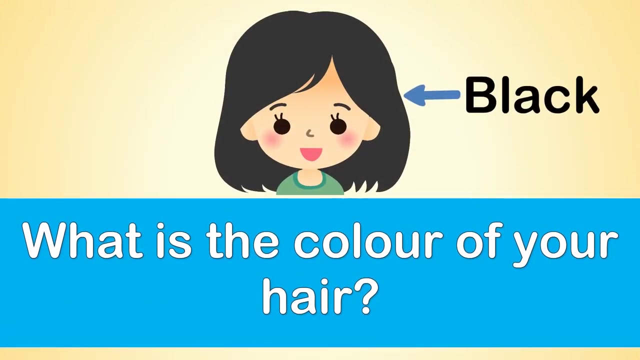 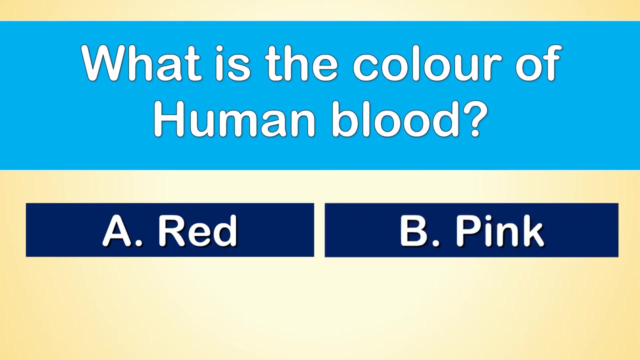 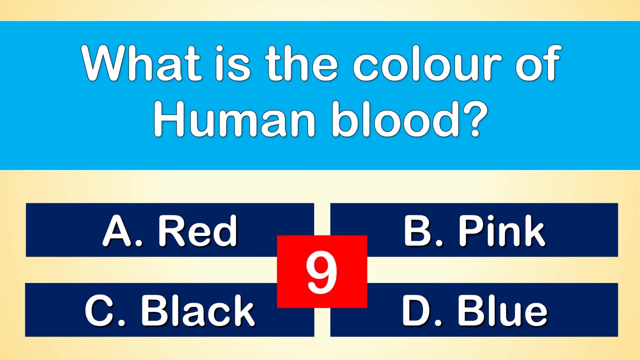 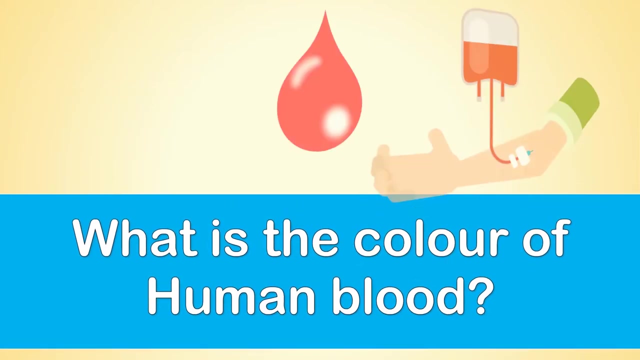 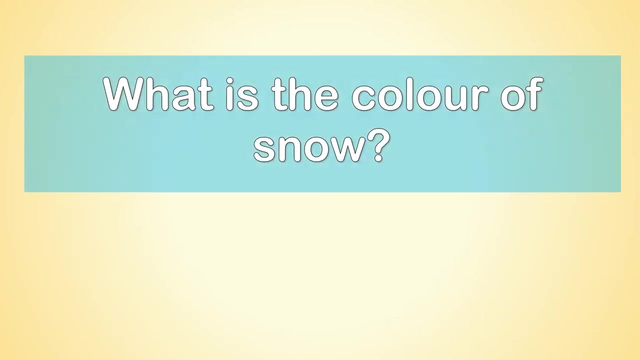 Quiz time: Color squeeze. What is the color of your hair? Red, pink, black, blue, Blue? Answer is black. What is the color of human blood? Red, pink, black, blue? Answer is red. What is the color of snow? Blue, white, black, green. 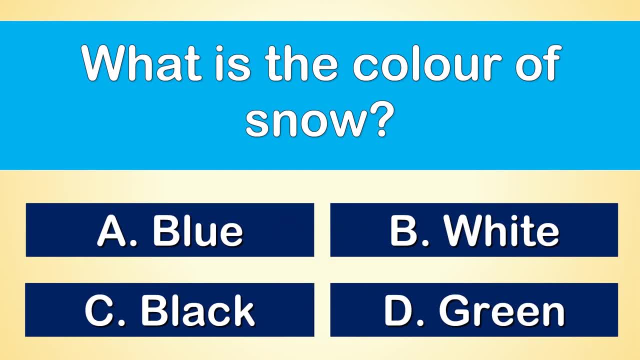 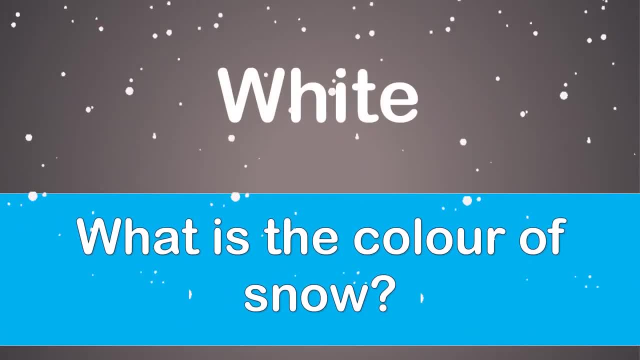 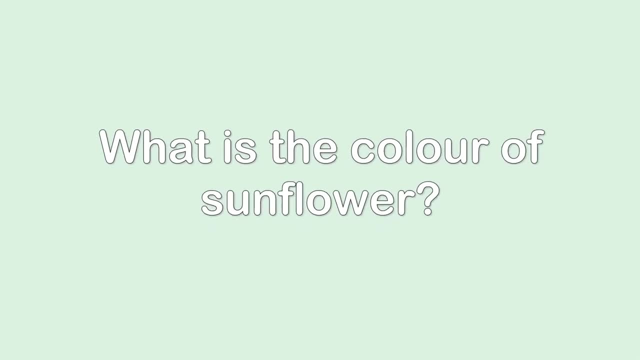 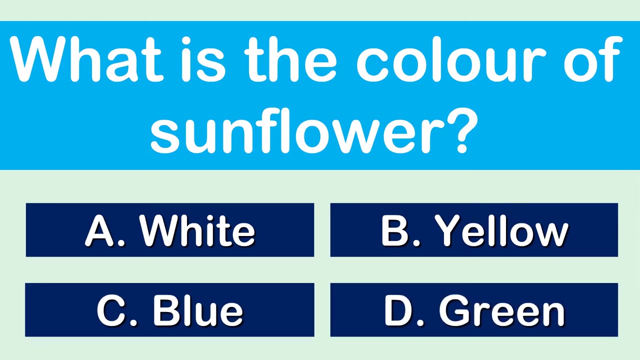 Answer is white. What is the color of sunflower? White, yellow, blue, green? Answer is yellow. What is the color of sky? White, yellow, blue, green? Answer is yellow. What is the color of sky? White, yellow, blue, green. 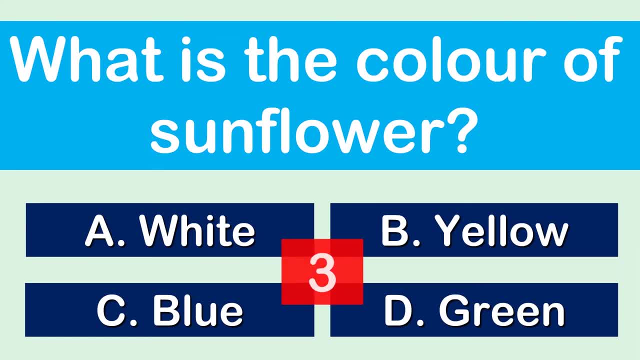 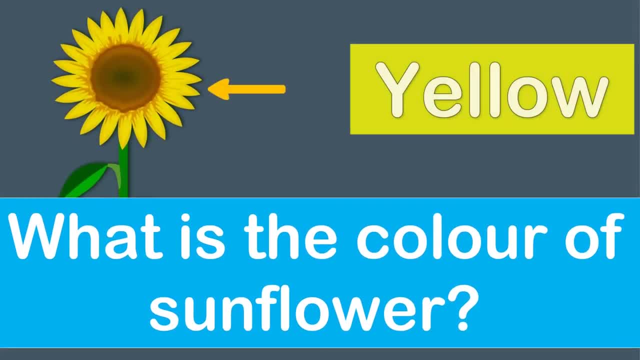 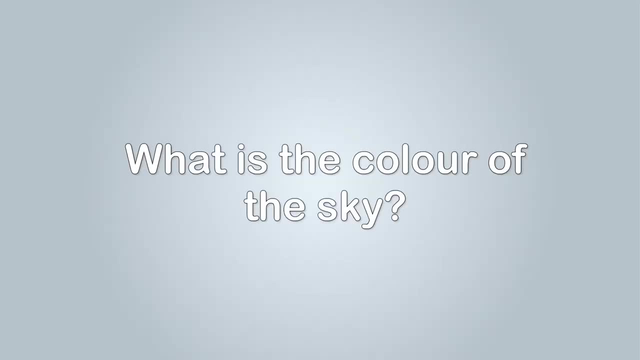 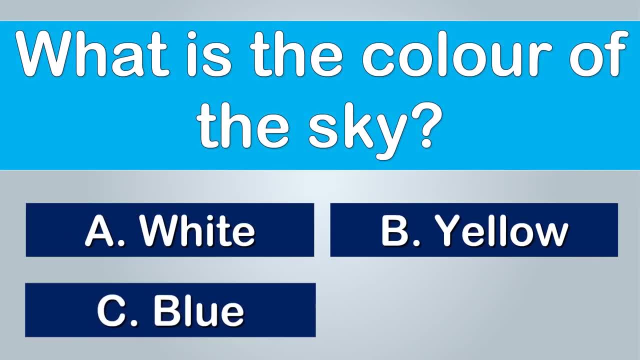 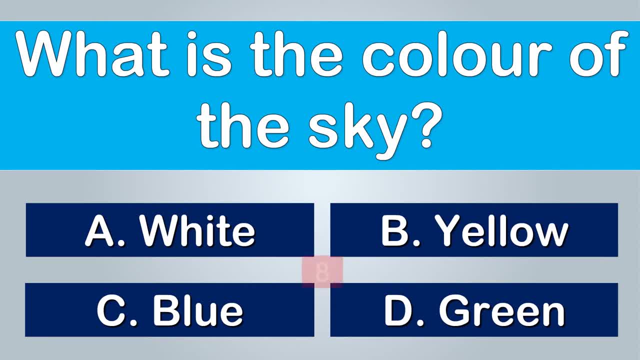 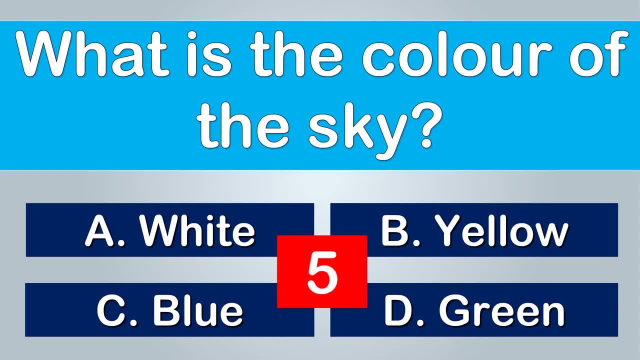 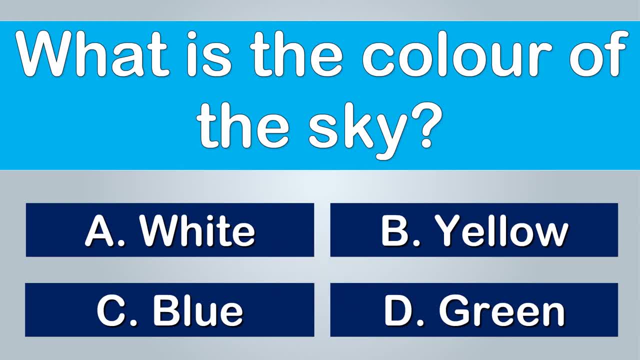 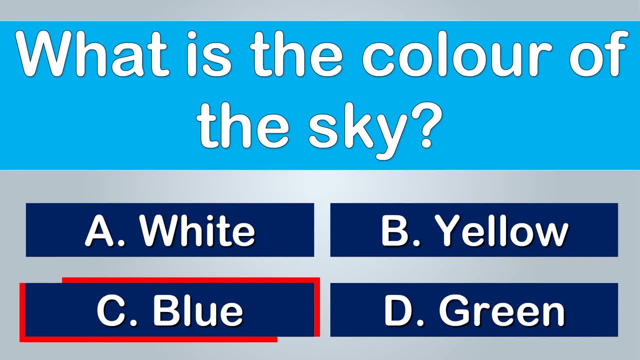 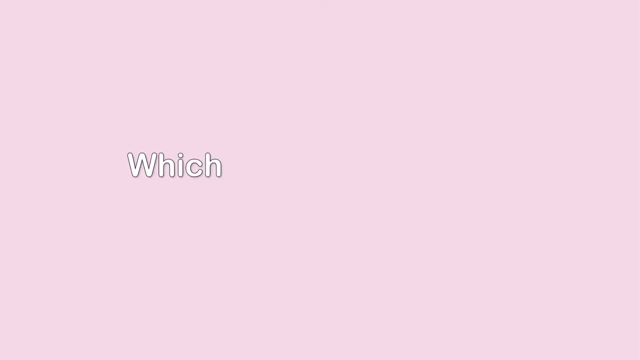 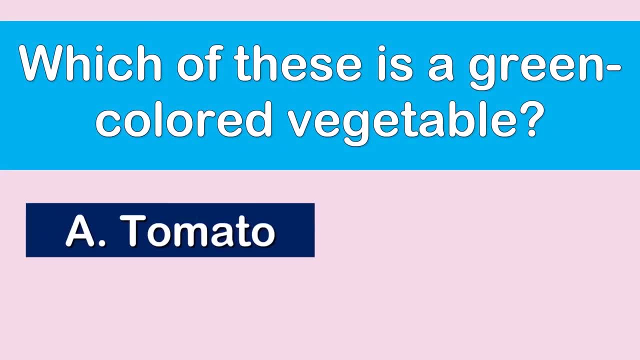 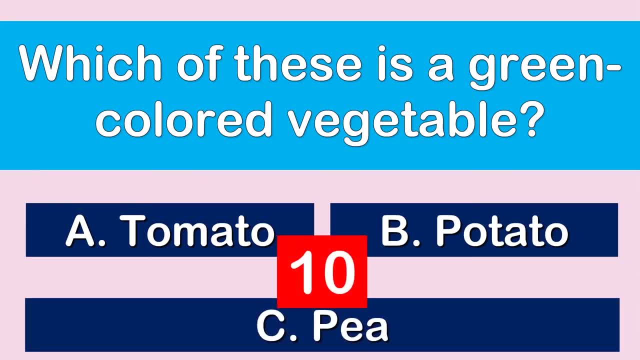 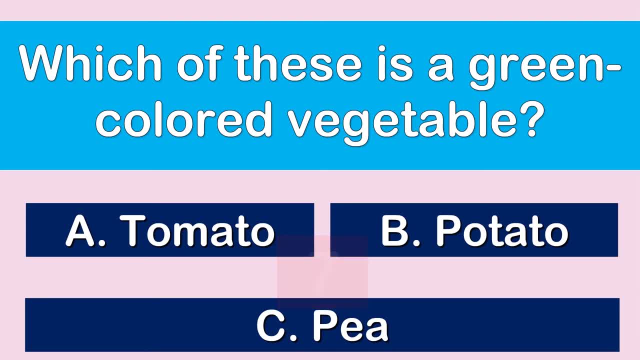 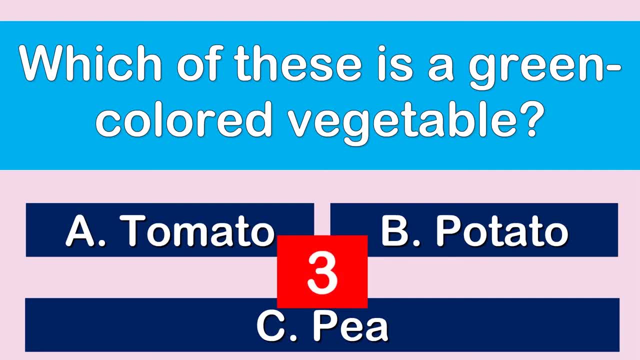 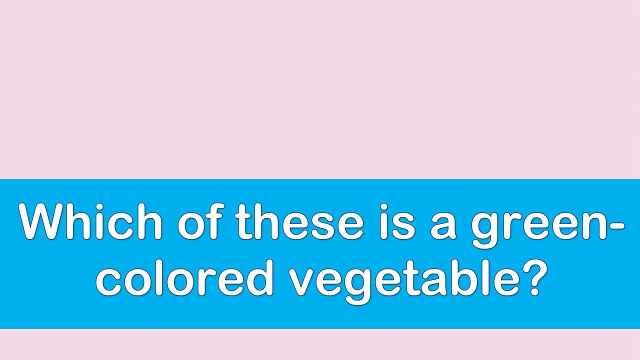 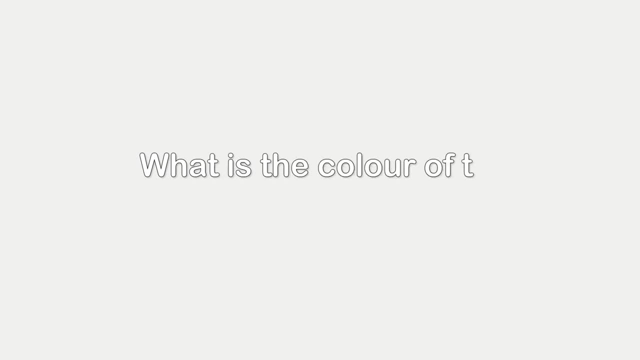 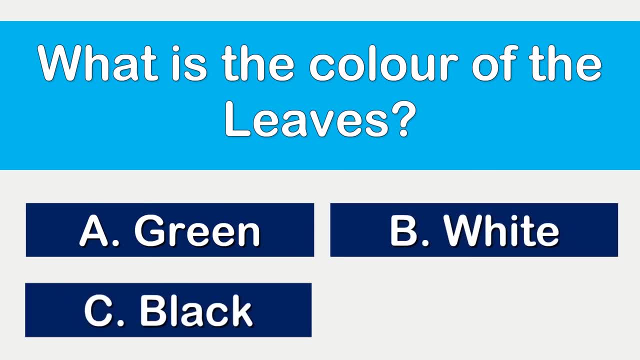 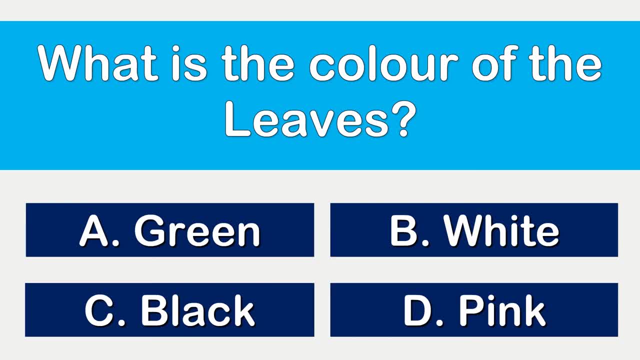 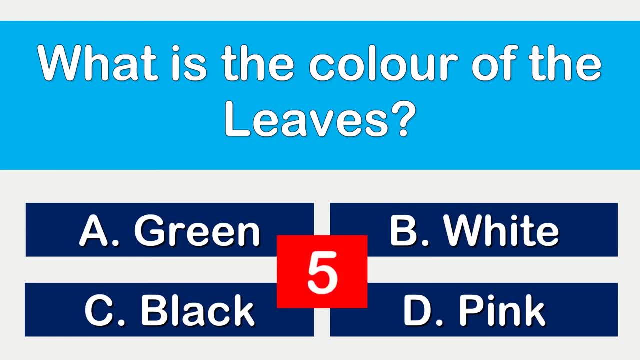 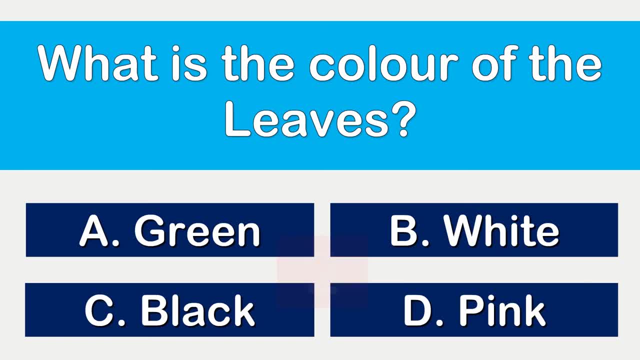 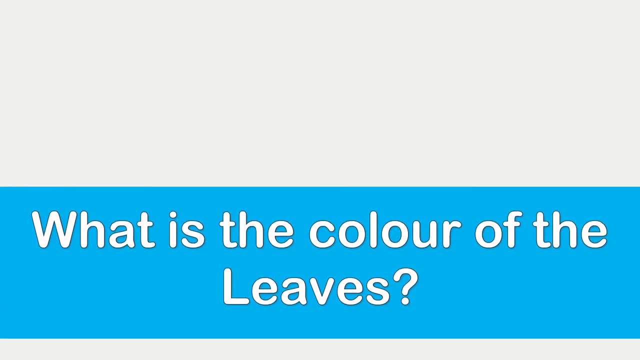 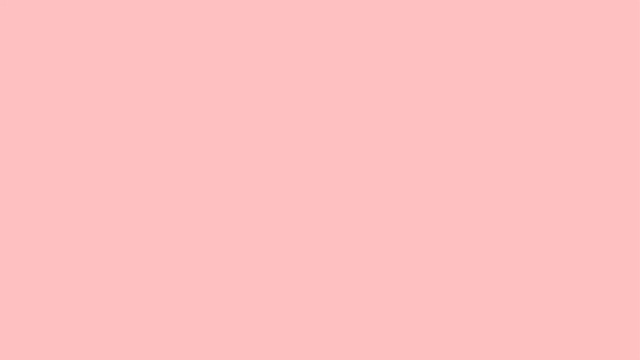 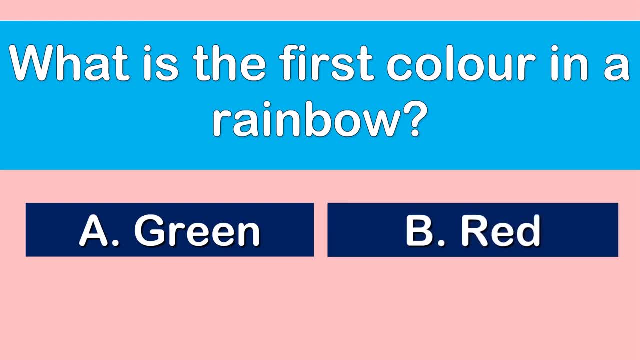 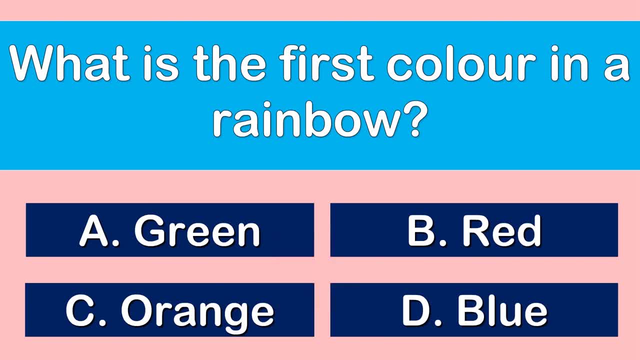 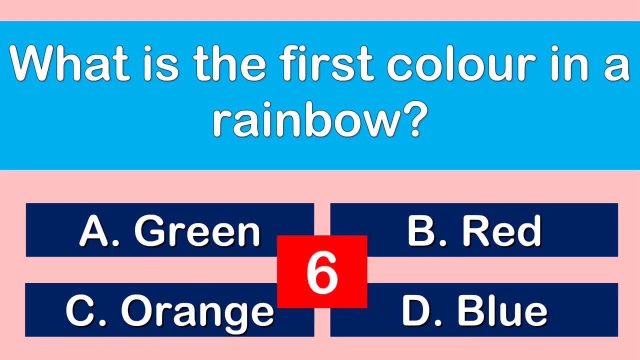 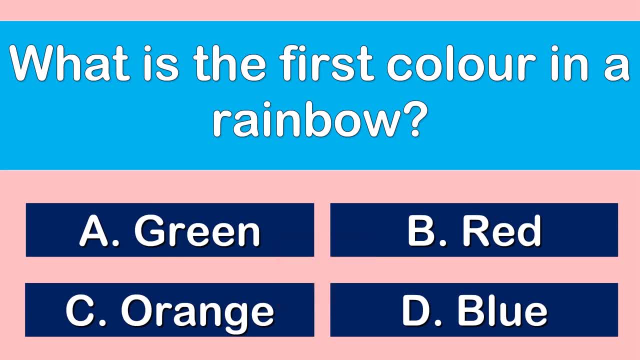 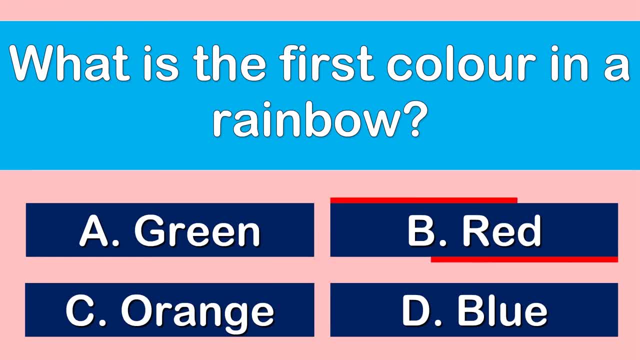 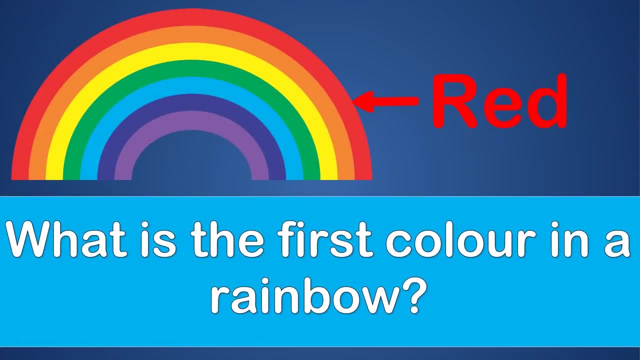 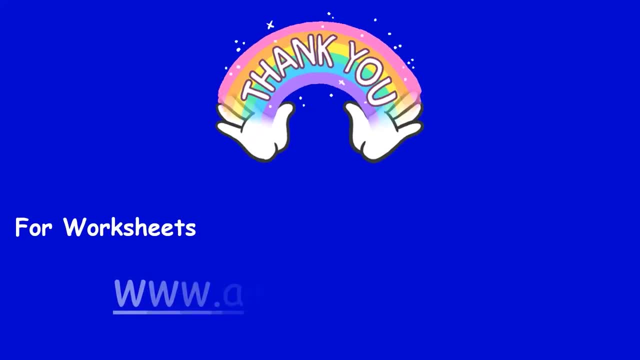 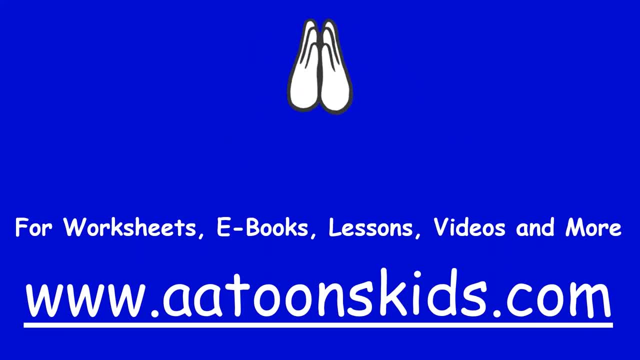 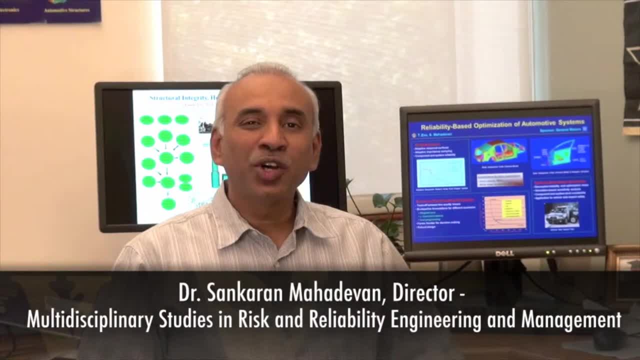 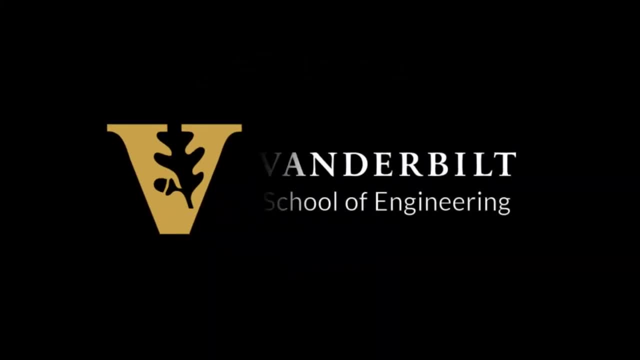 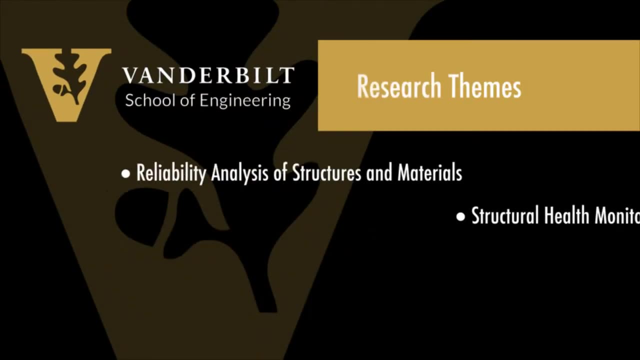 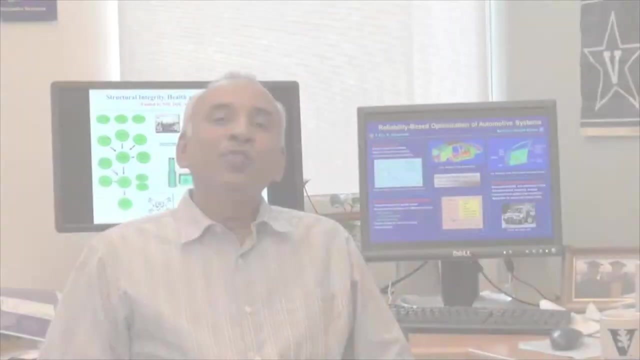 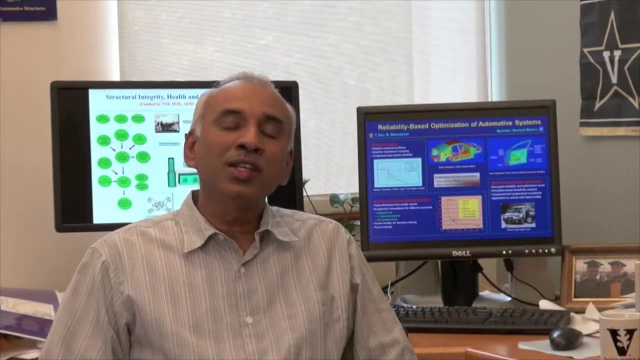 My name is Sankaran Mahadevan. I am the John R Murray Senior Professor of Engineering here at Vanderbilt. The fourth subgroup involves topics, which actually feeds into all the three subgroups, because this deals with model uncertainty. Now, all the three topics that I talked about: 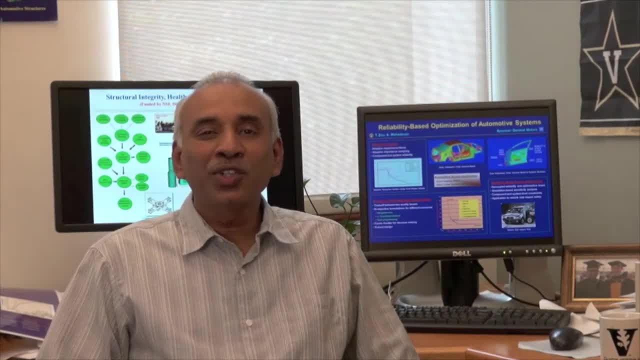 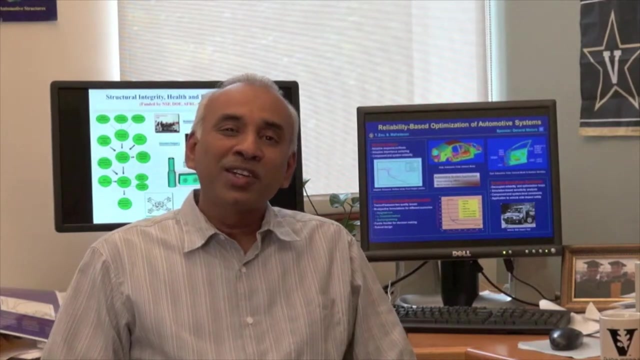 earlier, whether it was reliability analysis or structural health monitoring or optimization. they are obviously being done with computer models. So the natural question is: how good are your models? So that's the topic of this fourth group, model uncertainty or, in general, 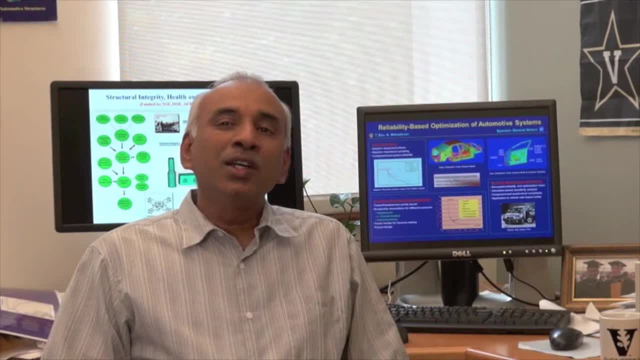 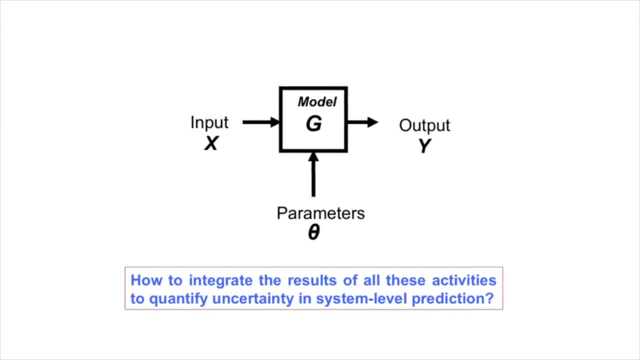 uncertainty quantification. So when we talk about uncertainty, there are several issues. One is, of course, if you take a system that you are trying to analyze, there are the inputs to the system. So you are trying to figure out. what are the uncertainties regarding? the